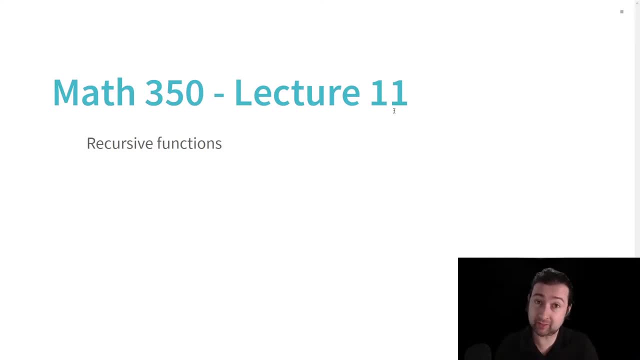 thinking about how to take a process that seems recursive and then actually implement it into code, And there's a particularly good problem on the homework exercises this week that I'm really looking forward to working through. So to begin with, we should think about or remind ourselves of: 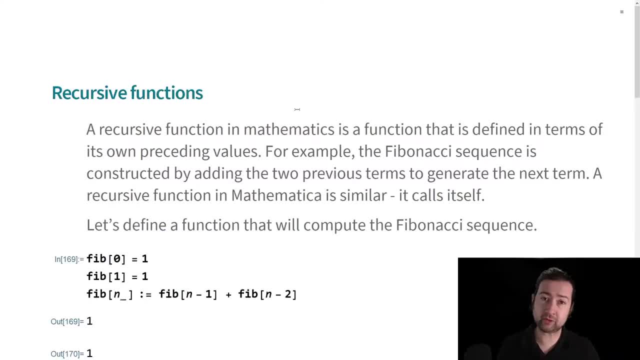 what a recursive function actually is. So a recursive function in mathematics is a function that is defined in terms of its own preceding values. So the first recursive function that most of us learn is the Fibonacci sequence, And you get the next term in the Fibonacci sequence. 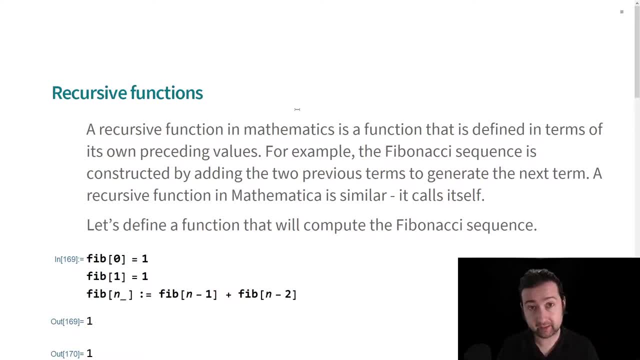 by taking the two previous terms and adding them together. Now that means that we have to have a starting point. So the Fibonacci sequence is the sequence defined, where the first two numbers are 1 and 1.. So once I have 1 and 1, I can construct the next number by adding those together to get 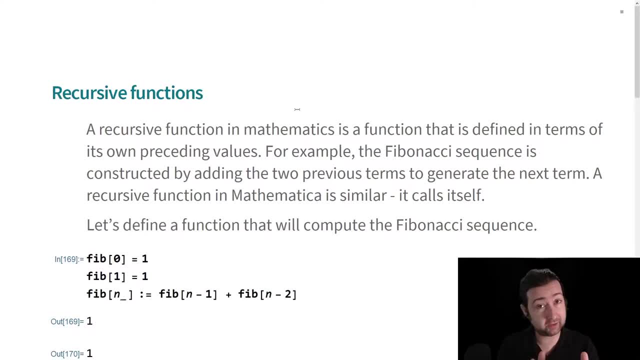 2.. And then I can take 2 and its previous term, 1, and add those together to get 3.. And then 3 and 2 is 5, and so on. So if we wanted to do this in Mathematica, we might take the naive approach. 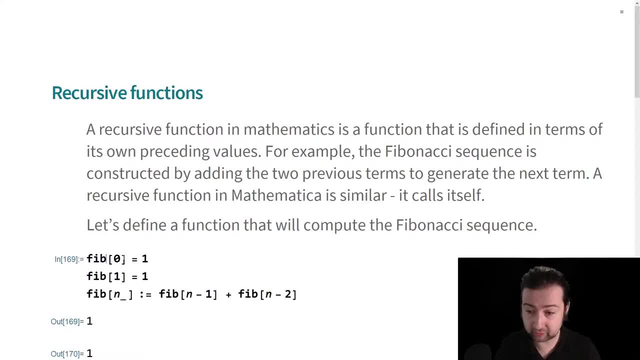 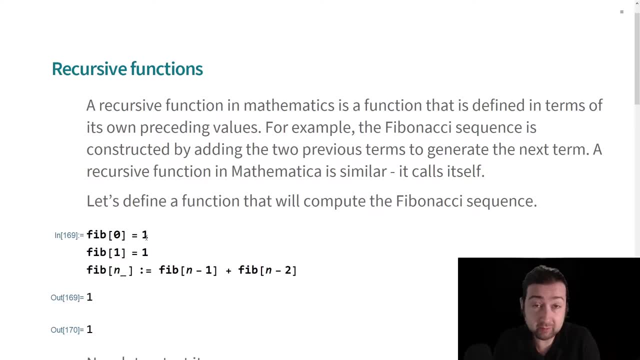 of just writing it and see if it will do it. So if we write down this function, fib, and set two initial values, because this function is going to require some starting place, So if we write down fib of 0 is 1 and fib of 1 is 1, then I've got a function now that I can. 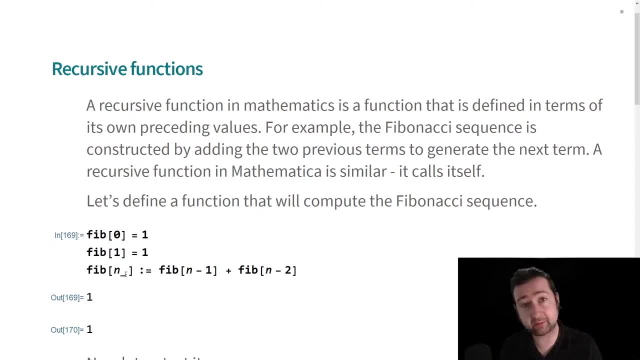 evaluate in terms of itself, And this might look weird, but this is a pretty typical structure in computer programming: to define a function in terms of itself And what it will do when you call it is it will look back at the previous function calls and then 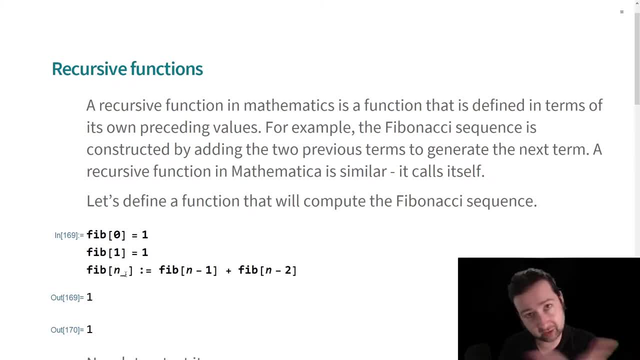 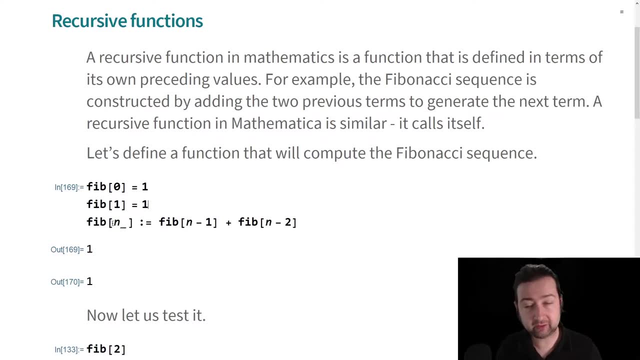 evaluate those, And if those have further calls inside of them, it will keep going backwards Until it finds something that it knows. So our function definition is that the Fibonacci fib of n is equal to fib of n minus 1 plus fib of n minus 2.. So let's test this out: The 1 and 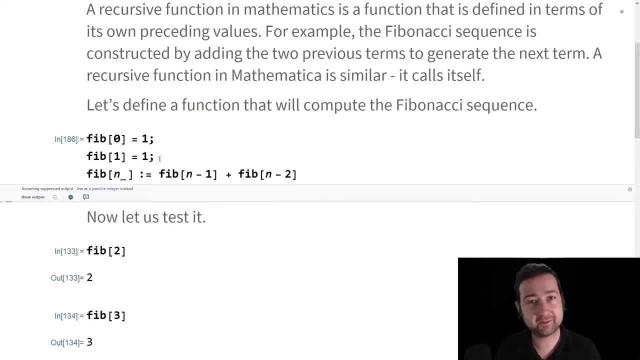 the 1 here came from the fact that I did not put my semicolons at the end of the values there. Okay, so let's test it. So, according to my formula, if I put 2 in here, well, that's going. 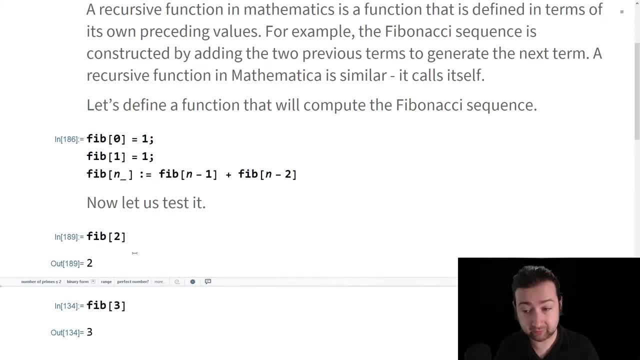 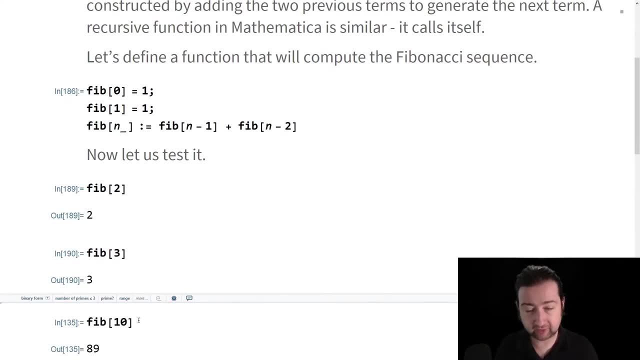 to call f of 1 plus f of 0,, which is going to be 2, because 1 and 1 is 2.. Fib of 3 is 3.. That's good, because 2 plus 1 is 3.. And I can keep going. I can test various numbers. 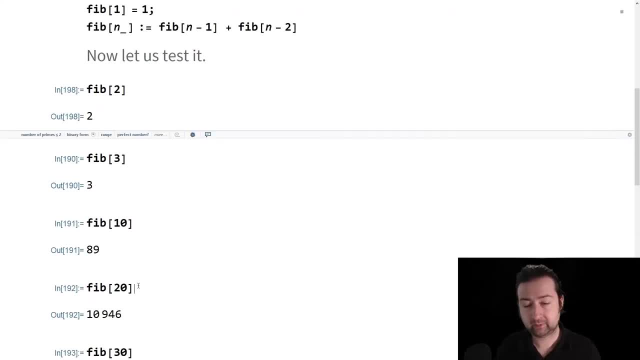 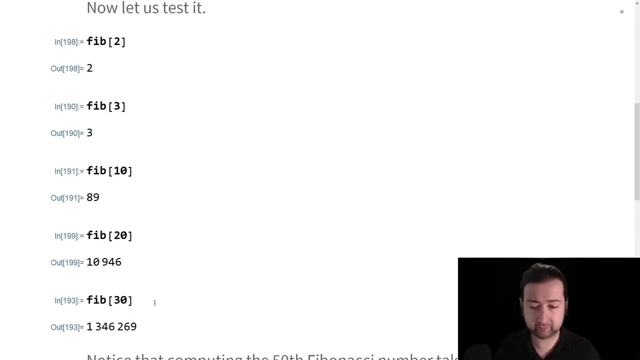 The Fibonacci of 10 is 89, so on. Now there's something you might notice. Maybe, since we're dealing with small values, you haven't seen this yet, But the problem, or not the problem, what you might notice- is that, as we evaluate larger and larger numbers, 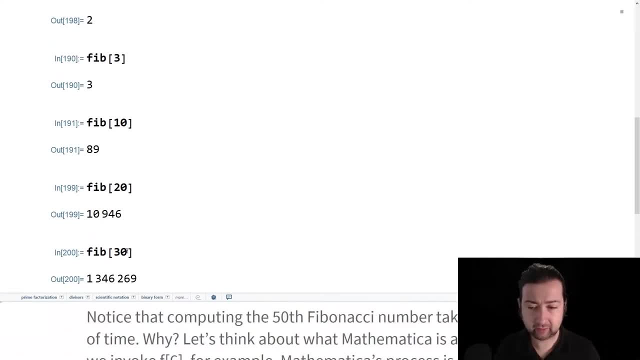 this program takes longer and longer to run. So if I put in 35 here, the program is going to take quite a while to produce the 35th Fibonacci number this way, In fact, it's still going. And you might think to yourself: why is it doing that? What is about Fibonacci of 35? 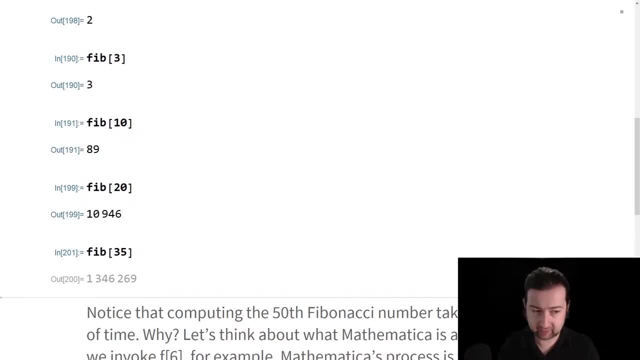 that's taking so long for the computer to execute And, yeah, we're just going to sit here and wait for this to finish evaluating, because there was a big difference between f of 30 and f of 35.. All right, so there is the 35th Fibonacci number. It's correct. 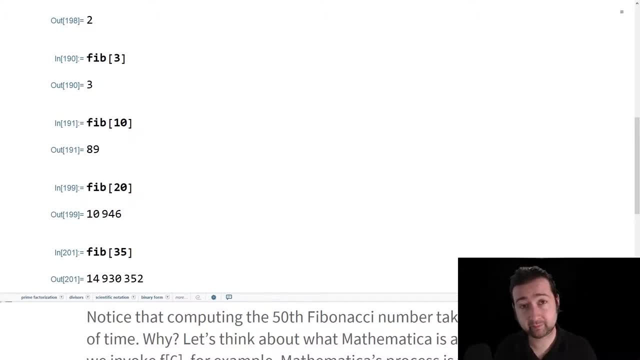 but that took 10 seconds to evaluate. So the question is: why did it take that long? The answer is that what Mathematica is doing when it calls Fib of 35 is it's evaluating that to be Fib of 34 plus Fib of 33.. So now it's got two things to evaluate. 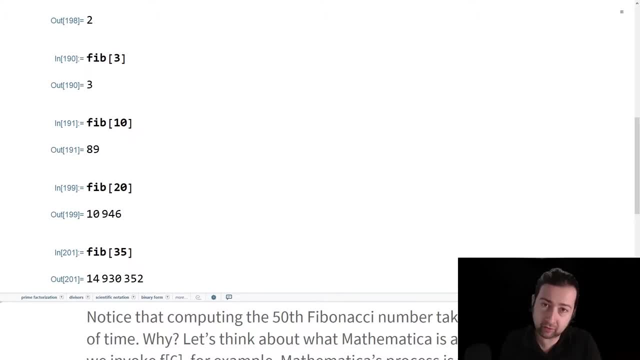 But then each of those has two things to evaluate And it doesn't know that it's already done some of the information that it needs to compute in one of the branches. So it recomputes everything at every step. So let me see if I can illustrate what I mean by that. 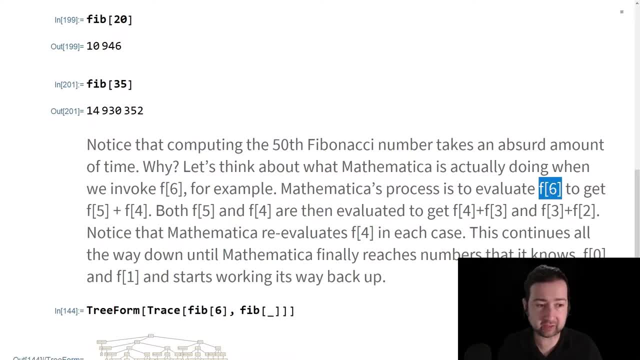 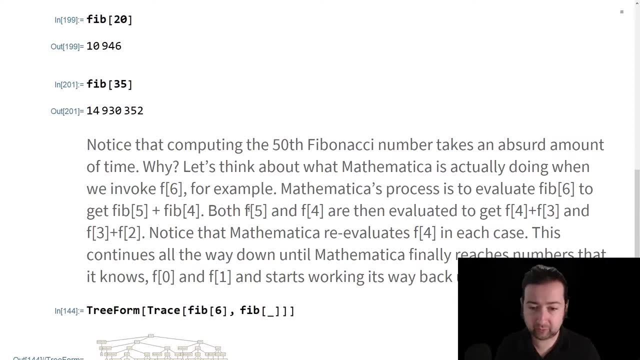 Mathematica's process, for example, say for a Fibonacci sequence of six, for fib of six is to get fib of five and fib of four. So now both fib of five and fib of four are evaluated. Notice though that fib of five is evaluated as the F of four plus F of three. 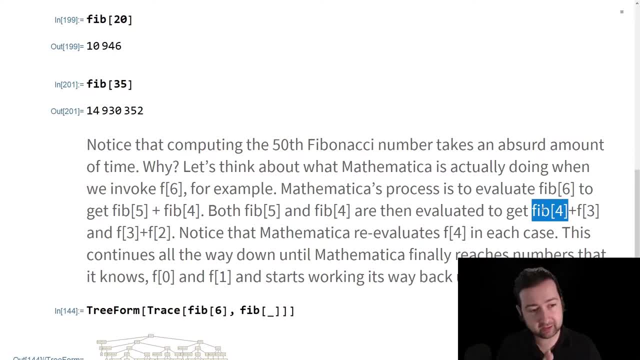 Well, it doesn't use the fact that it already evaluated this Fibonacci function at four to calculate this one. It redoes it, And so you get this huge tree of expanding cases where things are being evaluated over and over and over again, And this is not a way that a person would ever 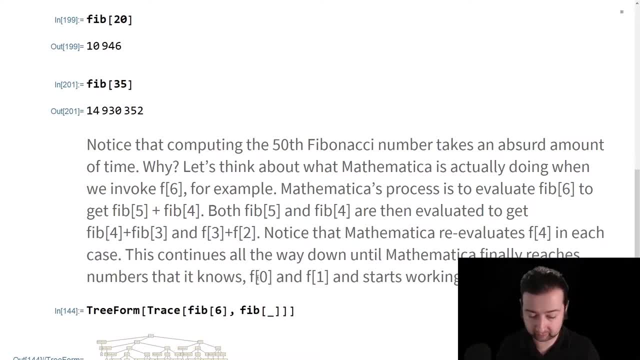 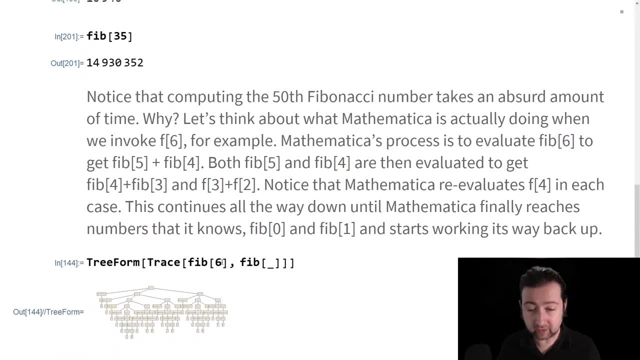 think to evaluate this. You would evaluate everything once, So we can actually see what's going on by looking at the tree form. There's a function here called trace that is going to be explained in the memoization notebook that accompanies this week's homework. I'm going to 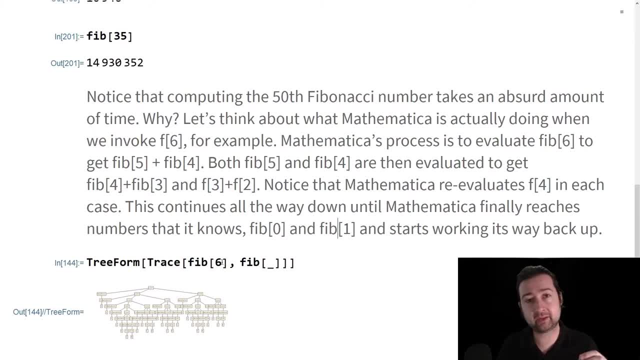 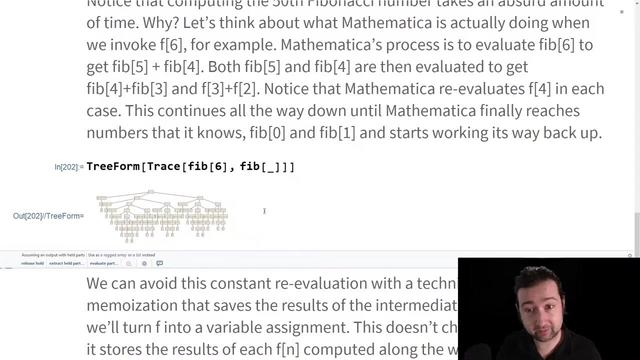 use it here and just tell you that what the trace function does is it looks at how a function is evaluated and it returns. So if you look at the tree form here, this is an enormous number of function calls that have happened. In fact, we can make this larger and you can see that that tree gets significantly. 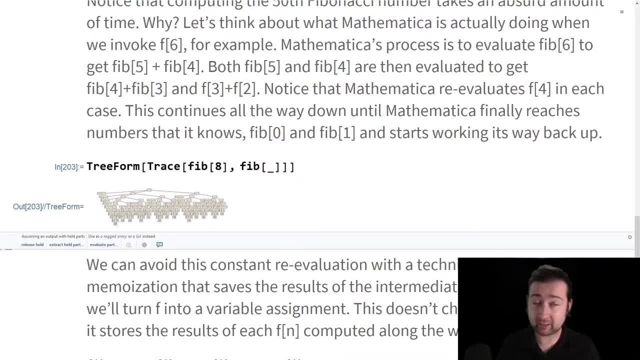 more complicated. So if you look at the tree form here, this is an enormous number of function calls that have happened. What you would expect to happen if this was acting in the way that a human did it, is that it would know that to get Fibonacci eight, it would have Fibonacci seven and Fibonacci. 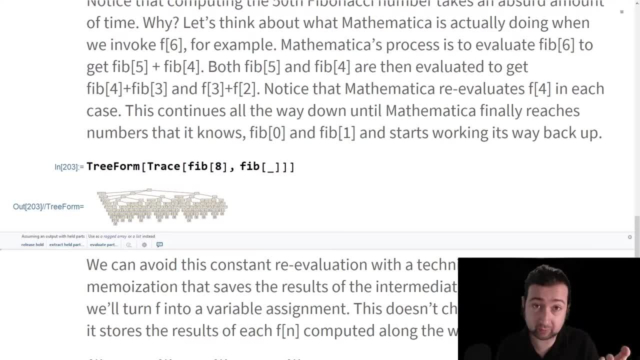 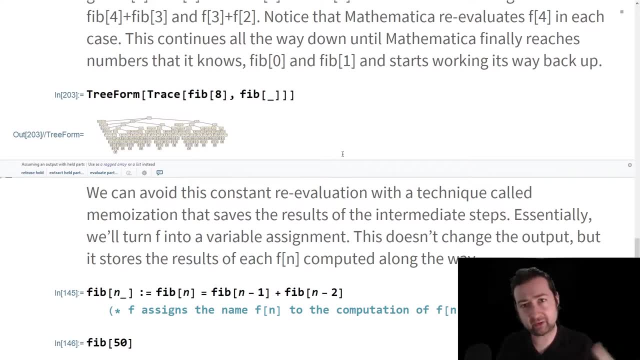 six stored somewhere so that it could just pull those numbers every time it needed to do a new evaluation. So you can avoid that constant reevaluation of Fib seven and Fib six and Fib five, which, if you're again in the memoization notebook, you'll see exactly how many times. 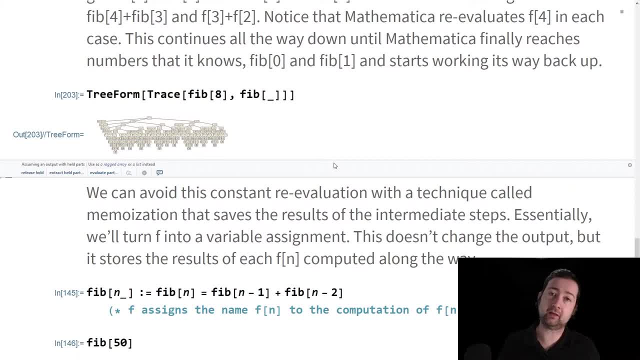 that's being reevaluated. It's completely absurd. So we can use a technique called memoization, which, for the purposes of this lecture, you should think of as storing the evaluations that have already happened, to make sure that mathematics can call them back up again when it needs them, instead of constantly reevaluating everything. 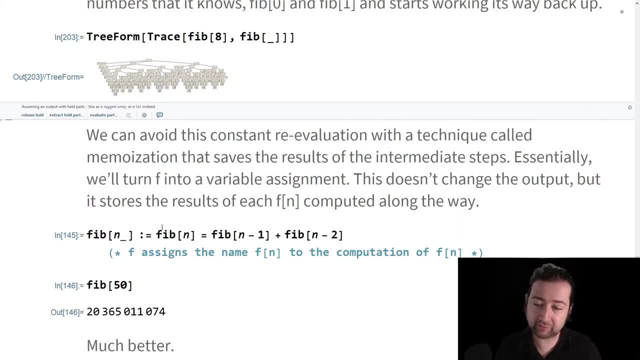 every time. So the way we can do that is when we define a recursive function, we can not only tell the function how to look at its previous values, but to actually store that information as well, with the correct label. Speaker 1. So this might look a little bit like a simple. 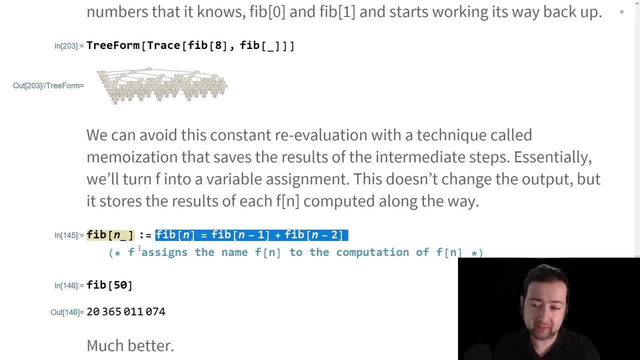 thing. It might look a little strange, but what this function is doing is it's defining Fibonacci of n to be a function assignment, a variable assignment. It says Fib of eight is equal to the assignment. Fib eight is equal to Fib seven plus Fib six. So that means that 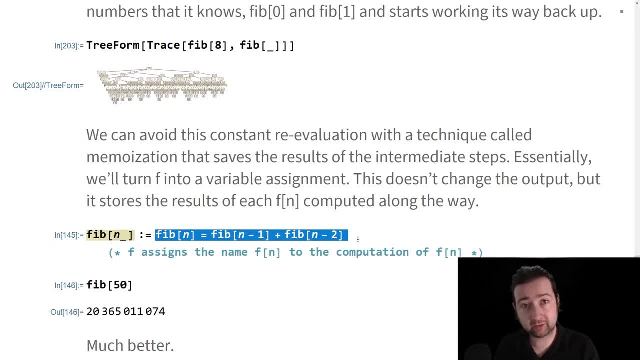 in the course of calculating what the eighth Fibonacci number is, it also records that number inside of something called Fib eight, And now mathematical will carry that around internally as a value it can refer to again, because the way that Mathematica acts is it always tries to call the most specific variable name it can find. So if Mathematica sees Fib, 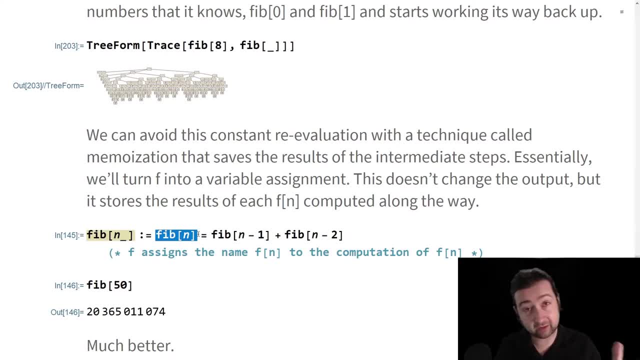 eight, and on the one hand it has a function definition that it can compute Fib eight with, but on the other hand it's stored something called Fib eight in memory. it will just pull the Fib eight from memory and use it instead of recomputing it. So now, it took a long time. 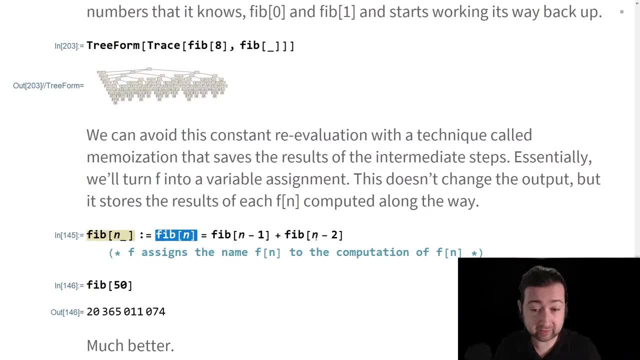 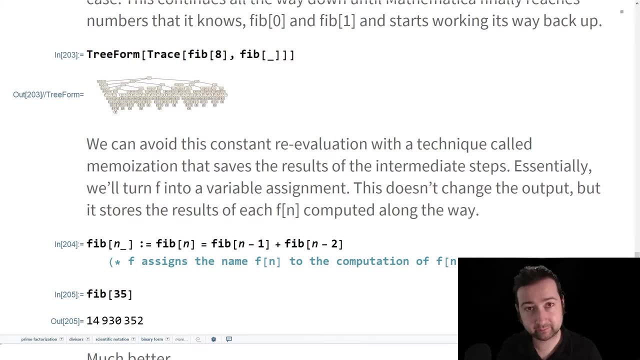 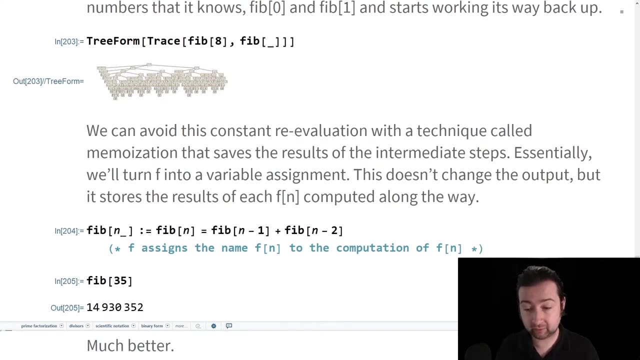 to compute Fib 35.. This will be our redefinition of the Fib function. And now let's compute it again. Well, that was almost instant. Okay, So, and all of the values between Fib one and Fib 35 are now sitting in memory. Of course, we can check that by looking at the command. what is stored? 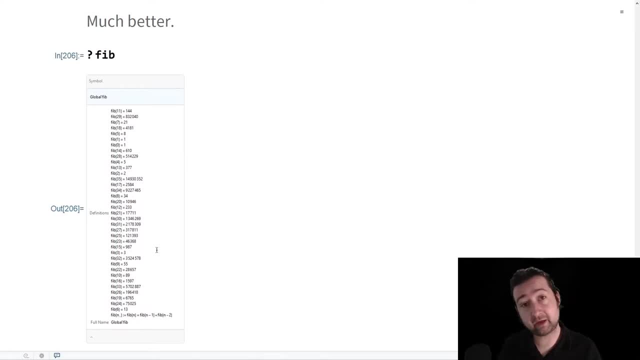 inside of Fib. And you can see, this is the trade-off that we've made. We have traded speed for memory. So now Mathematica is carrying around in memory all of these values of the Fib numbers that it can just call on when it needs to. 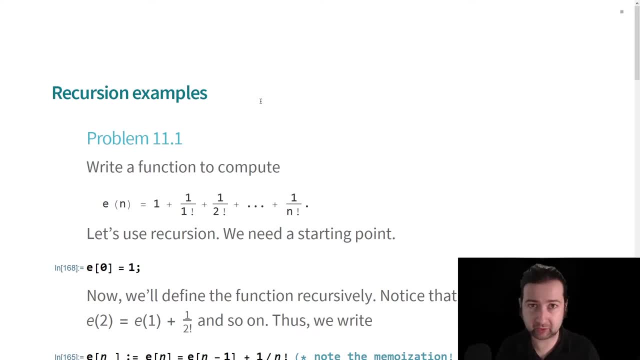 So let's look at some examples of recursion that are not just the Fib sequence. So the first thing is, let's look at an example- We've actually computed two different ways already- which is a function to produce the sum of one over the factorials, And this is called. 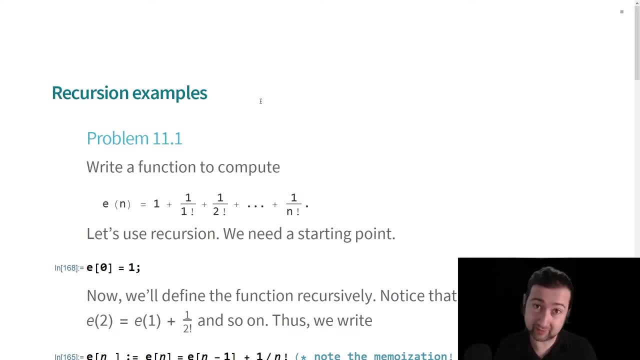 en, of course, because this sequence ends up converging to the number e in the limit. So if we're going to set something up as a recursive operation, then we need a starting point always. And the way I'm going to think about this function is: well, the zero value was equal. 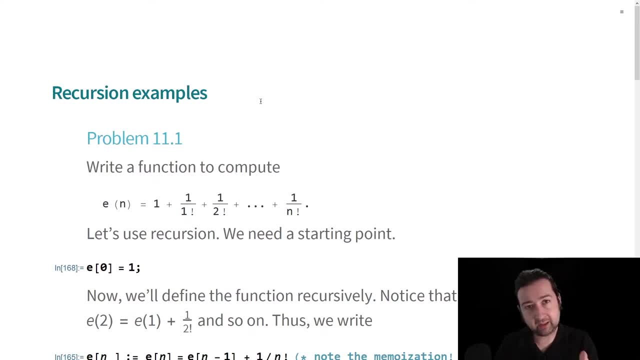 to one, and then I get the next number in the sequence by taking the existing number and then adding one over n factorial to it. Okay, So I look at the previous en and I add one over n factorial And that's what I'm saying here. E2 is, or sorry, E1 is E0 plus. 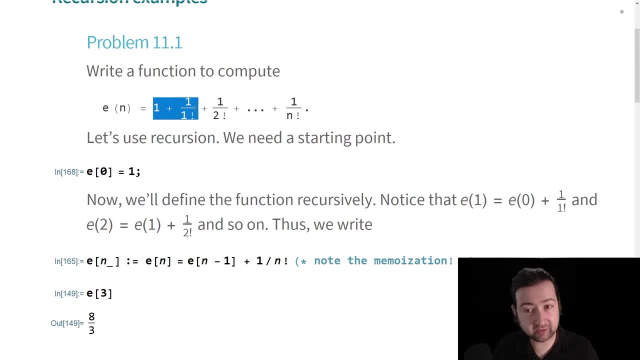 one over one factorial. E2 takes E1, which was this bit right here- and adds one over two factorial to it. En is going to take En-1.. which is all this, and it's going to add 1 over n factorial to it. So we're going to write. 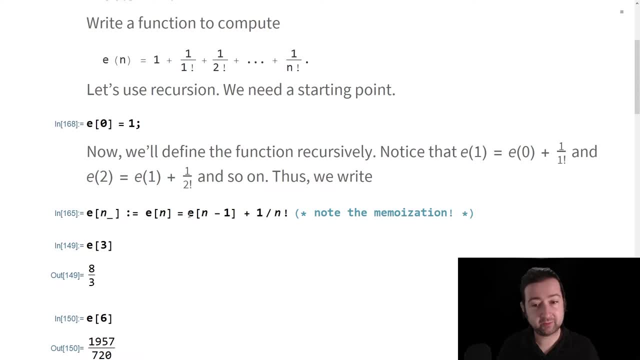 en is equal to en minus 1 plus 1 over n factorial, And notice that I've used the same memoization trick here to make sure that this runs efficiently, where my definition of the function is not just a calculation, but it's going to do the calculation and then also store it in a name so it can be. 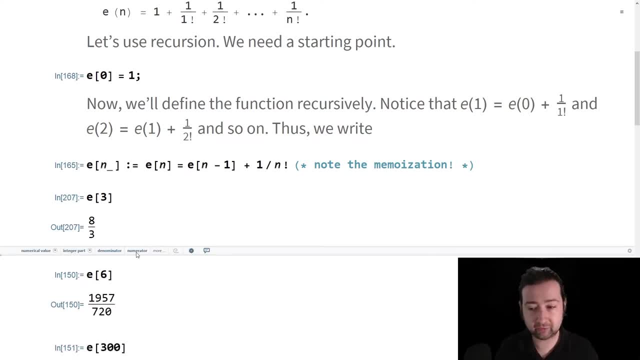 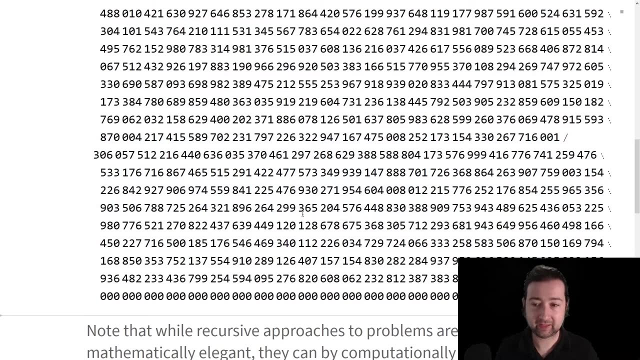 recalled when necessary. So you can compute this if you like, for large values of e and so on. e of 300 is a large number. I'll show all of it so you can see it. It's a pretty big number. It's a. 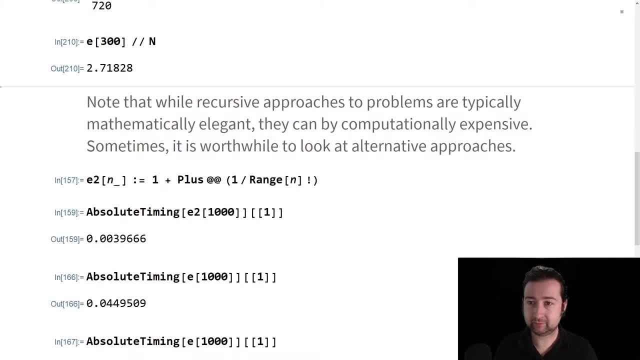 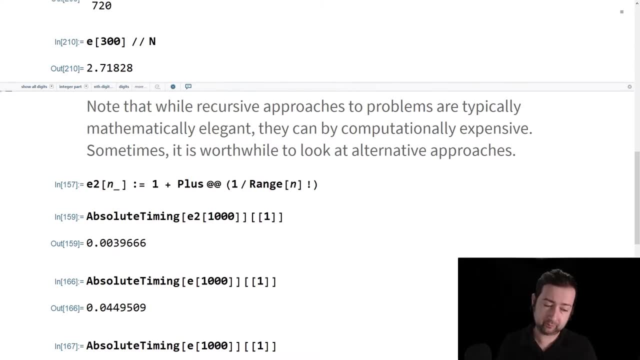 fraction. So actually I'm curious here what this is equal to. Oh, that's starting to get pretty close to e at this point. So one thing to notice about one thing that you might run into when you're working recursively, is that Mathematica actually has an internal limit on how many. 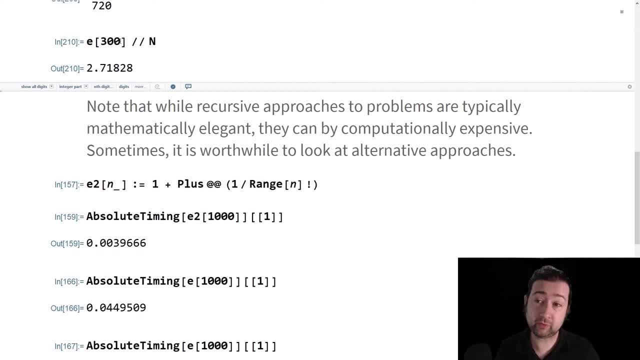 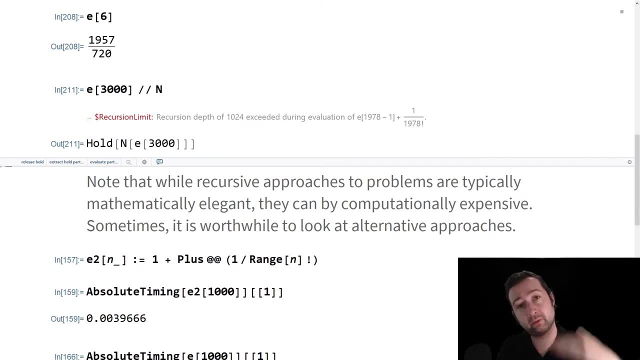 recursive steps it will take Before it quits. So if you tried to evaluate this command at e 3000, it's going to tell you that it's hit its recursion depth, which means that it will not run this more than 1024 times And it 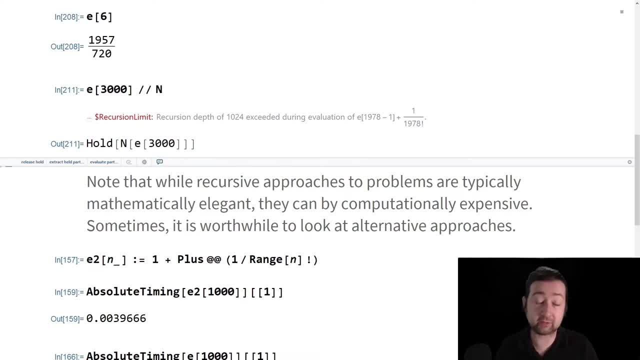 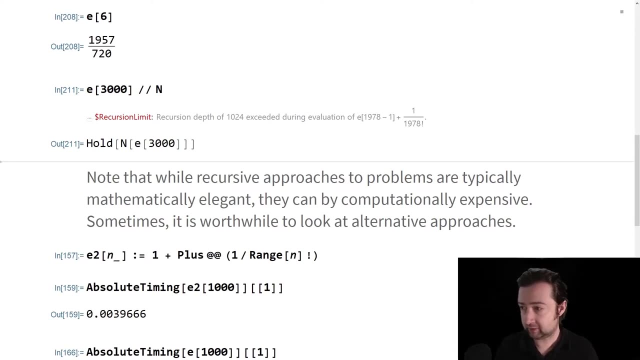 does that as a hard barrier against out of control processes, which are easy to do when you're doing recursion. If you want to go further, then you can redefine the recursive limit to whatever you want it to be. So the appropriate response to something like this would be to redefine. 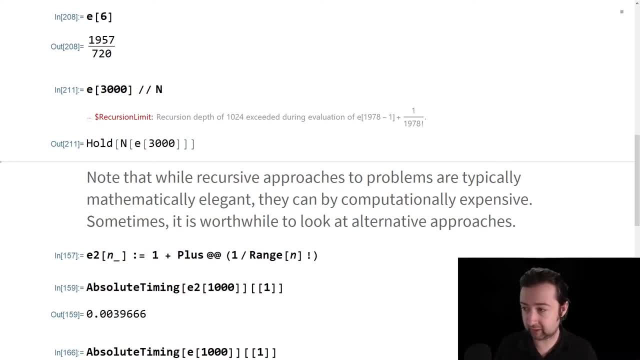 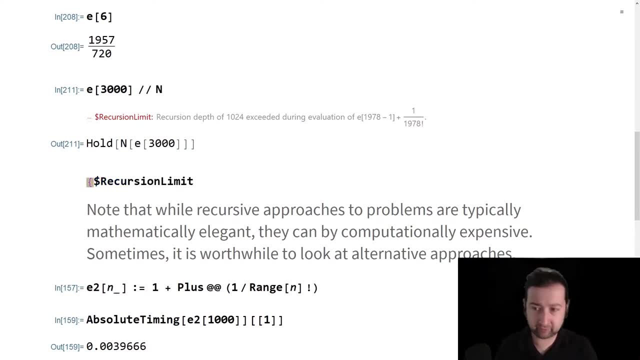 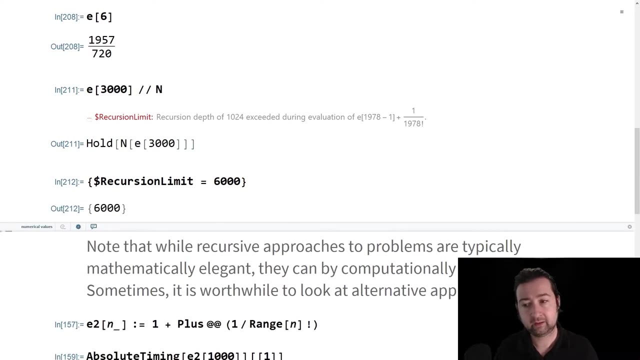 what's called the global variable in the following way: So any global variable in Mathematica can be set with a command that looks like this: So we're going to take the recursion limit variable and we'll reset it to say, I don't know, 6,000.. Now, having done that, we should be able to run this. 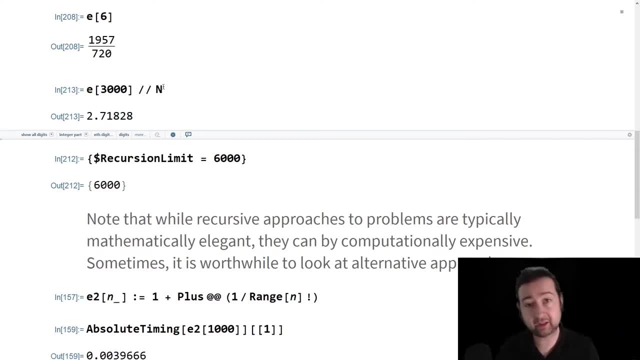 command again, And now it will produce our number for us, because at this point it'll recurse 6,000 times instead of the 1,024 times that it's set by default. So just an option that you should be aware of when you're looking at these things. A thing to keep in mind is that when you're 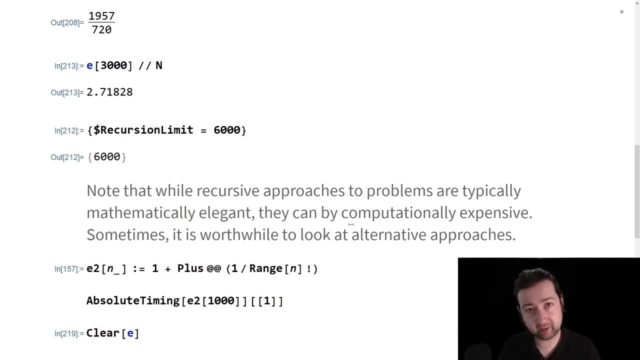 approaching a problem recursively, that oftentimes that's a mathematically elegant way of thinking about how a problem works. The issue is that computing recursively tends to be more expensive than computing directly, at least the first time through, Once you have built out a bunch of cases. 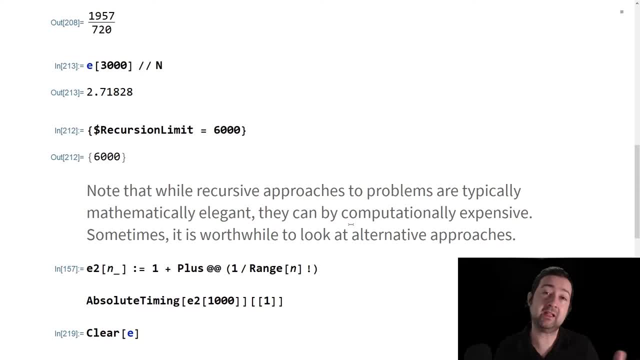 using a recursive function and you've stored those values, it's very easy to refer to them again, And so there's a trade-off here between an explicit function that can always just compute a value based on an input and a recursive definition of a function that is very fast once it's computed all the values once, but is a little bit slower. 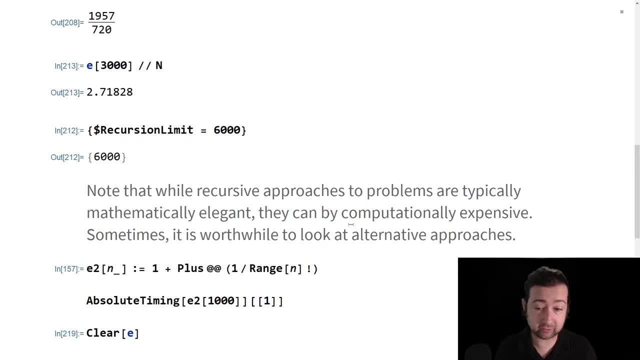 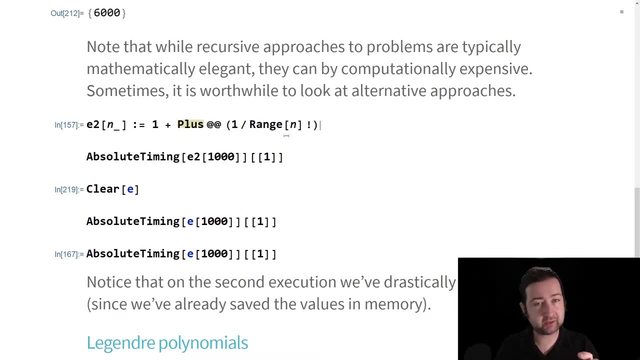 if you're computing a value for the first time And I want to illustrate that. If we define a new version of the function e with this 1 plus, the plus applied to 1 over the range of n factorial. that's the same function, but from a list-based approach where we take the range 1 to n. 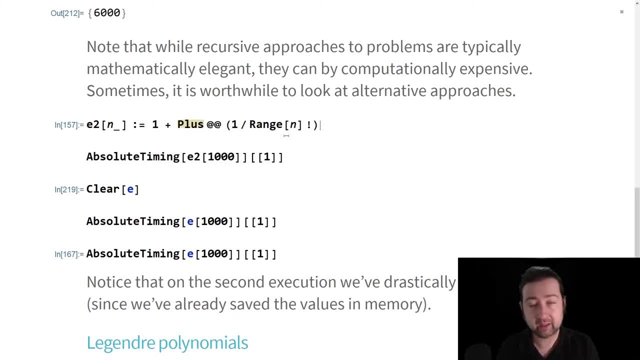 we factorial it, we take 1 over that and then add all those together. That's an explicit way of computing this function. e? n. So if we do that and we hit it with this absolute timing function, an absolute timing gives you an output that the first entry is how long the function took to. 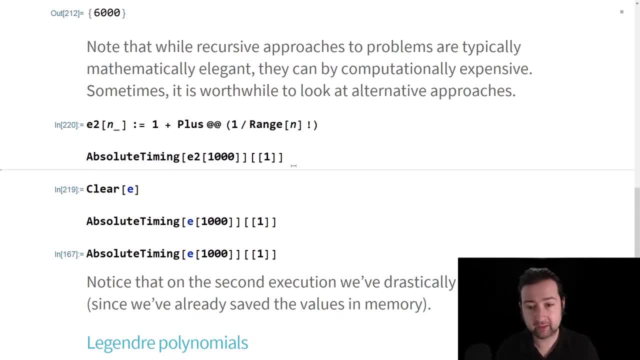 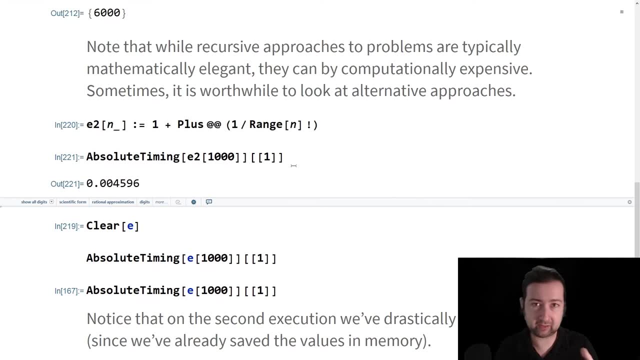 execute. and the second entry is the output of the function. If we do the absolute timing of this function running once on an input of 1,000, we see that we've got a function that's got 0.004 of a second. So 4,000th of a second is about how long that explicit function took to. 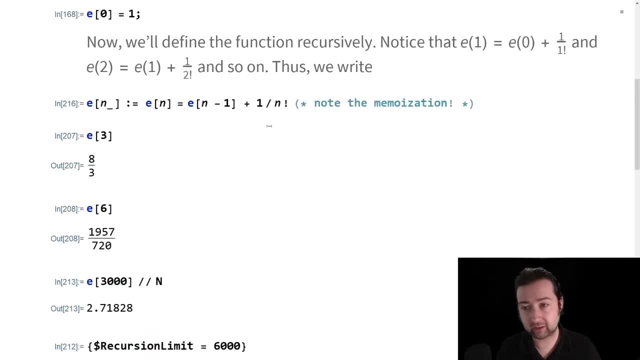 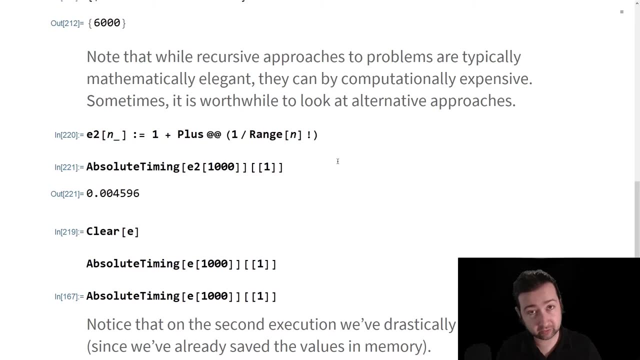 run. Now I've cleared the definition of e so that I can feed it back in again, And the reason I did that was so that I don't have the values pre-stored, because I want to compare how long it took to run the first time to the second time, The first time that we run our function with an. 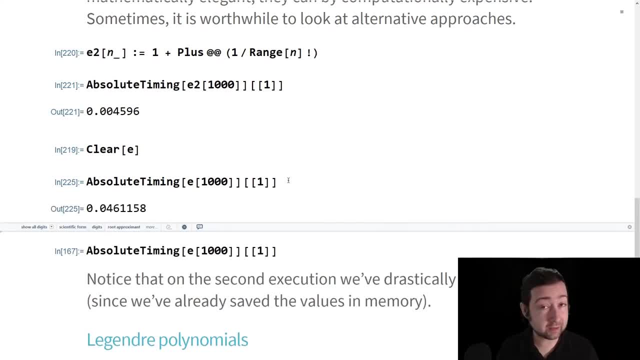 input of 1,000, you can see that this has taken 10 times longer to run on the first go. So this is four hundredths of a second that our function took to run, versus 4,000th of a second, And that difference is going to get even more. 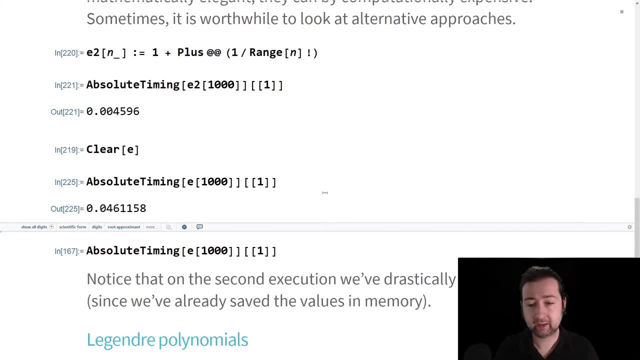 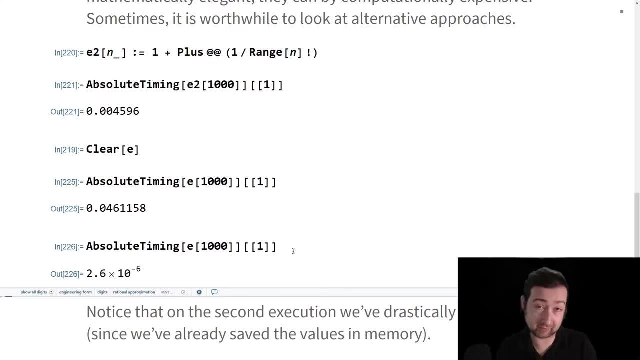 pronounced as the input gets larger and larger. However, the second time we run it, it has all those values pre-stored in memory. So the second time through, it takes a millionth of a second to produce a number, as opposed to the thousandth. you know, 4,000th of a second. that we've got right. 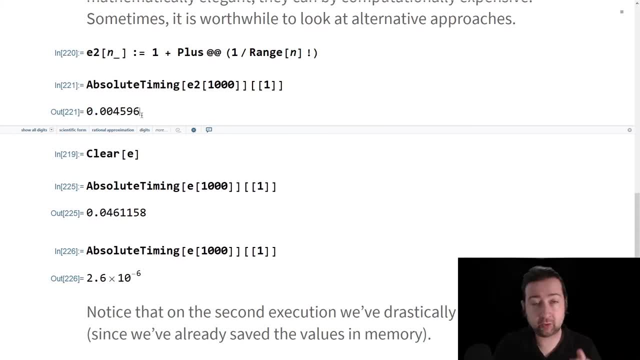 here. So there's timing issues to think about when you're working with recursive formulas versus explicit formulas. Also, the trade-off between running a recursive formula once and getting a table of values that you can refer back to, in which case that function is going to be very fast if you're having to use. 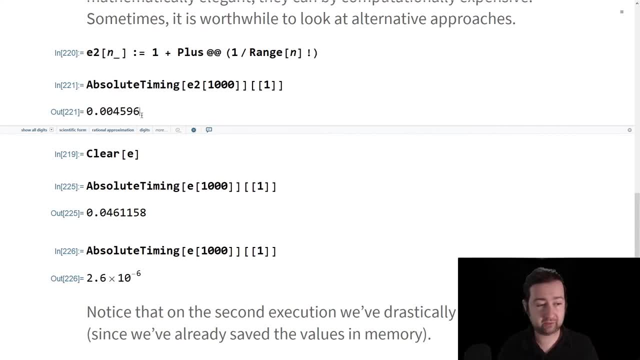 it over and over again. So the big trade-off that you're making when you're using recursion and you're memoizing is that you're trading speed for memory. So we're having to store things in memory to make them fast. This used to be a way bigger concern in the days when computers had 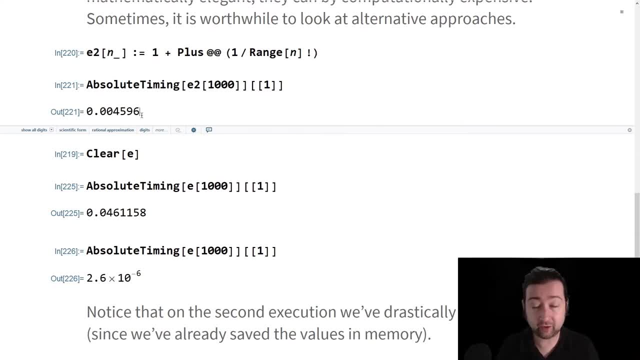 very, very strict limits on the amount of memory they had available. Now, basically, you can think of memory and storage, as free Computers have enormous amounts of RAM and enormous amounts of hard drive space, And so it's very easy in most cases that you're going to deal. 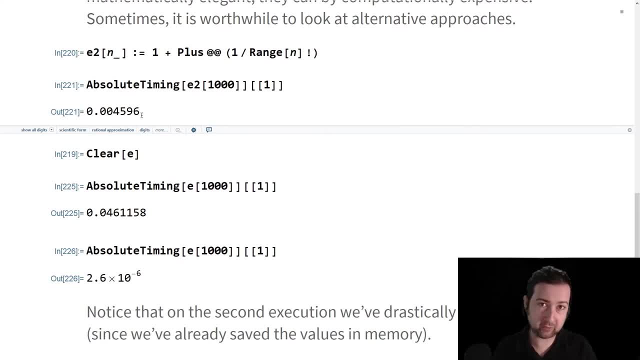 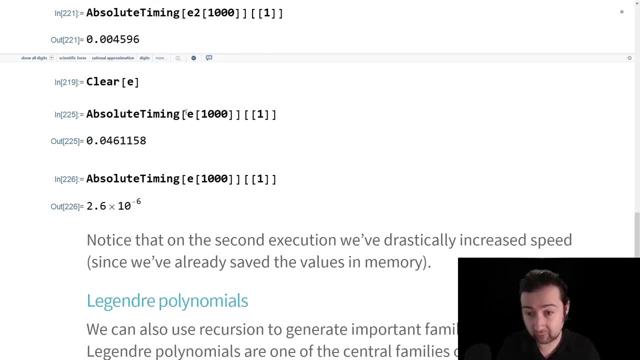 with, as a mathematician, to trade speed for memory in a way that's not really going to cost you anything, because we have so much free space available in memory. So right now what's happening is this function E is holding a thousand values of E in memory as a table. 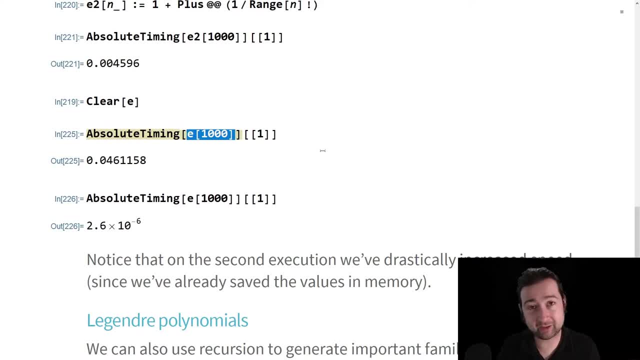 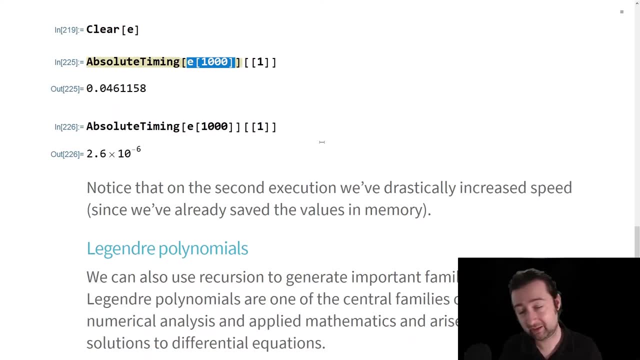 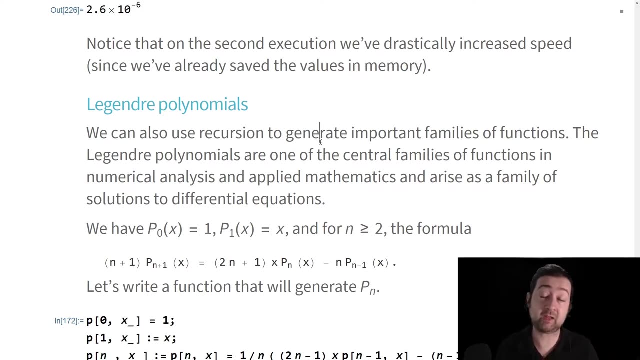 but it doesn't hurt anything because, I don't know, my computer has 24 gigabytes of RAM inside of it, right, And way more hard drive space than that. So another interesting place that you can use recursion that shows up frequently in applied mathematics is in the generation of special. 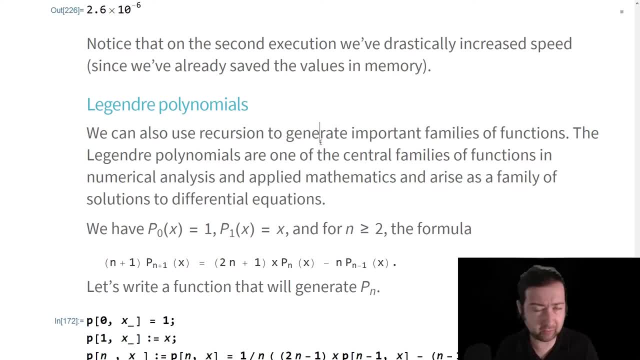 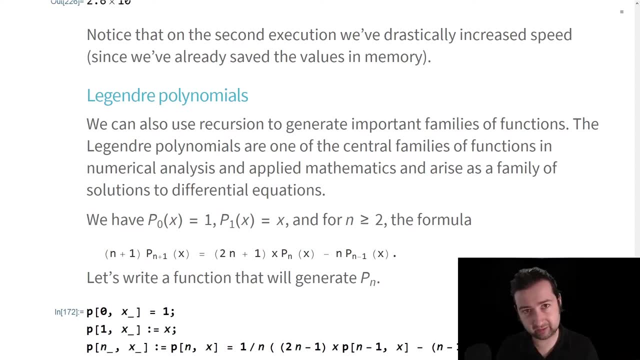 families of functions, And recursion is an equally good way of looking at the generation of functions as well. So one of the most important families I've picked one. there's, you know, six or seven of these that I've picked, And I've also picked one that I've picked, that I've picked, that I've 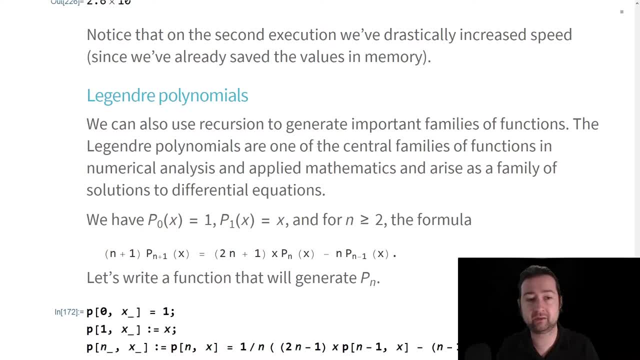 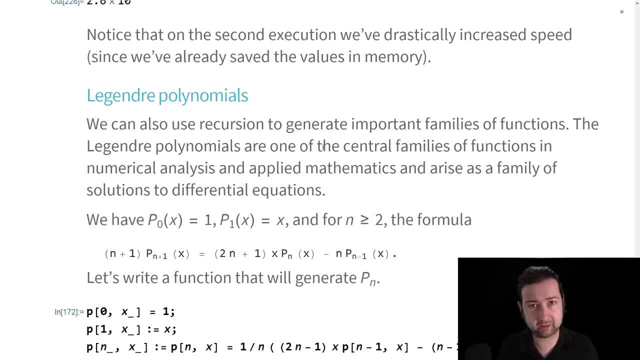 are one of the central sets of polynomials that show up in applied math, So you can use them for approximation theory, for example, and they show up in a lot of applications of physical systems as well. One of the ways to define the Legendre polynomials is as the 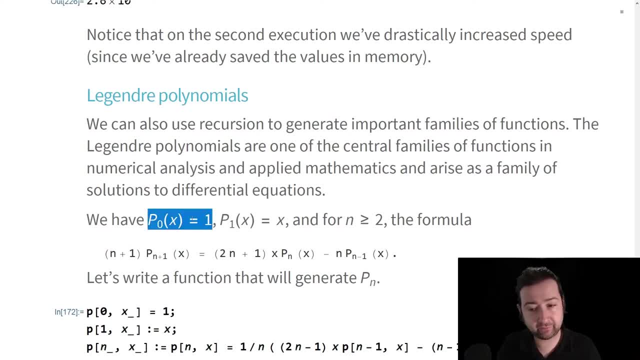 output of a recursive relation where you start with the first the Legendre polynomial being equal to one and the second Legendre polynomial being equal to one. So I found that a lot of polynomial being equal to x, And for n greater than or equal to 2, you have a formula that looks: 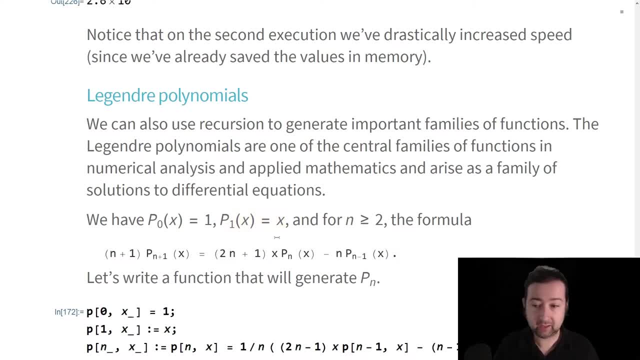 like this that defines all of the rest of them. Okay, Now we want to write a function that generates pn, but not just that generates pn. We want it to generate pn and is still a function of x, That is, we want to be able to work with it as a function. We want to be able to plot it. 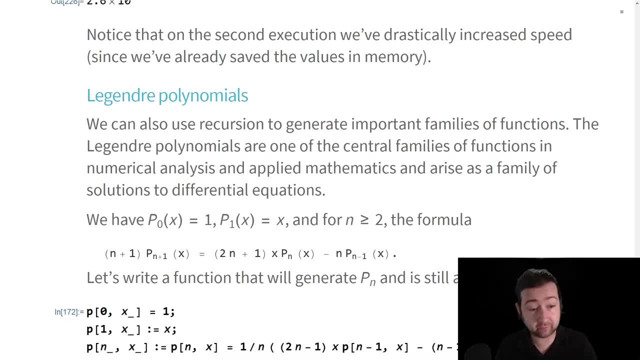 to do numerics to it. We might want to integrate it. We have to multiply it by other functions, So I need to make sure that it remains a function of x. And the trick that you use to do that is, when you set up your definition of your recursive function, you actually explicitly make the things. 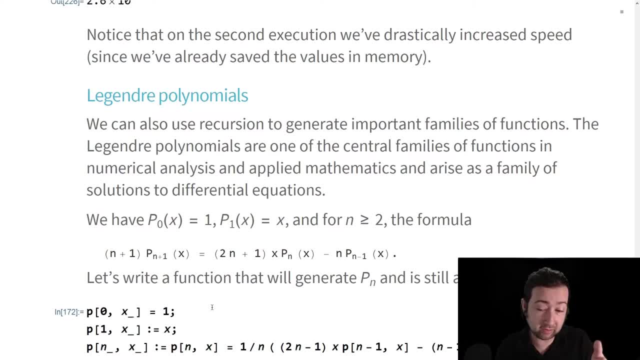 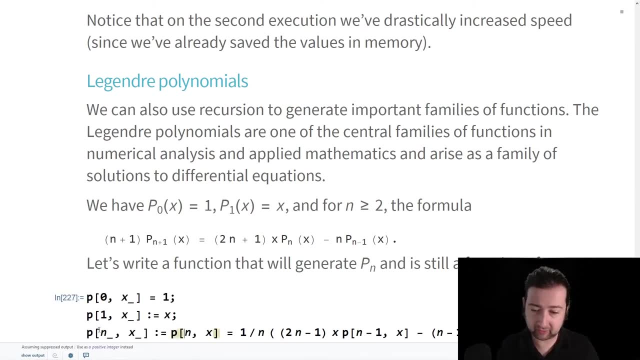 that you're building functions of x. So p0 of x is 1, p1 of x is equal to x, And then for the remaining values, what we're going to do is we're going to use this relation right here, And I don't. 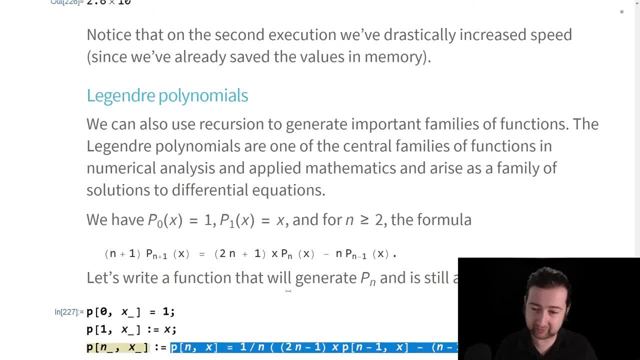 want you to get confused that this is different than this. All I've done to get from this relation to this function is shifted the index of n by 1, and then I divided both sides by 1 over n. So it's the. 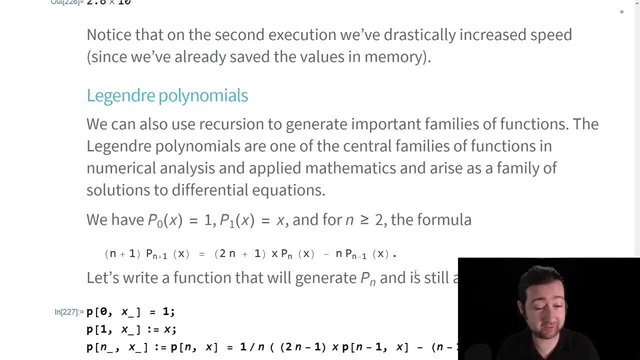 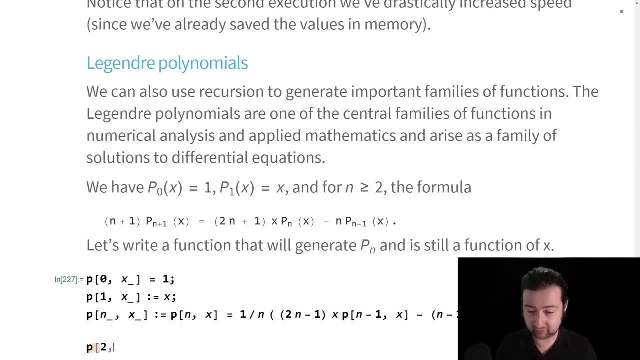 same relation, but converted so that a computer can handle it. So let's actually take a look at some of the values that this thing might spit out. Well, what is p, say 2 of x? That's a good thing to look at, And I happen to know that that is the second Legendre polynomial. Okay, 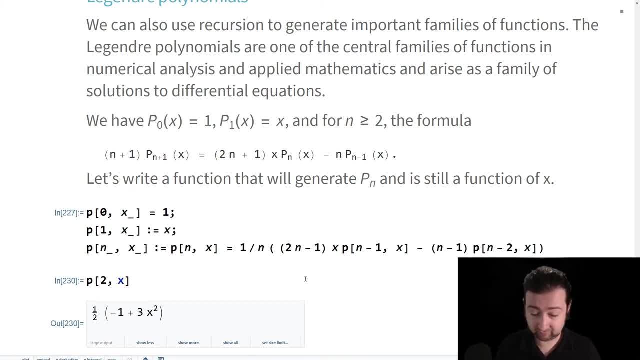 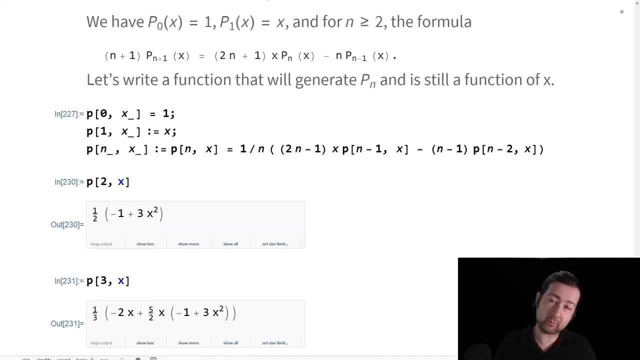 you can go look that up in a table if you like, And we can look at p3 of x. Now, one property that Legendre polynomials are supposed to have is that when you integrate them in product that you get zero out, as long as the Legendre polynomials are different from each. 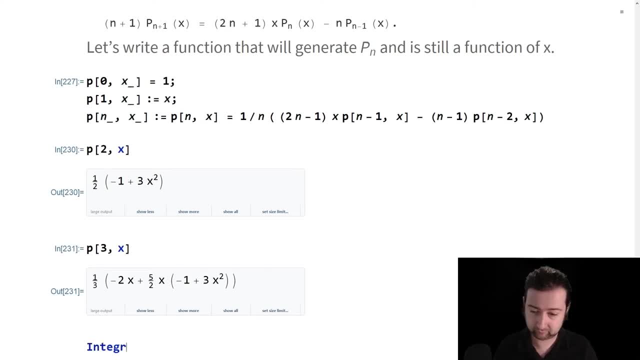 other. So let's integrate p, let's see the product of, I don't know, p2 of x and p3 of x, And then the interval that we're going to integrate on is any symmetric interval, but let's just do from minus 1 to 1.. 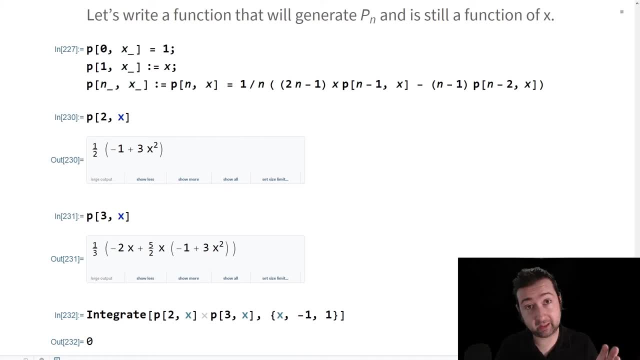 And we get 0. That's perfect. That's exactly what we're supposed to get. And notice that, even though we defined it with this recursive relation, we're getting actual functions of x out that we can work with with calculus ideas. So these are functions. 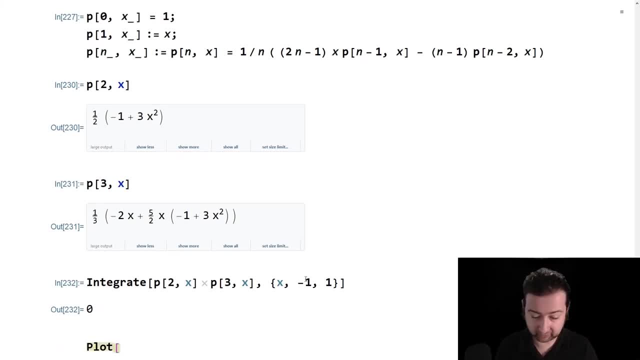 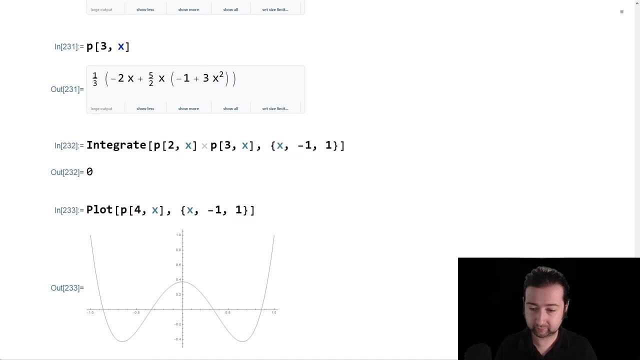 If you're not convinced, we could plot them. So let's plot p4 of x From. x goes from minus 1 to 1, right, That's exactly what we'd expect to see. In fact, one trick that you can use here is we could show lots of them at the same time. 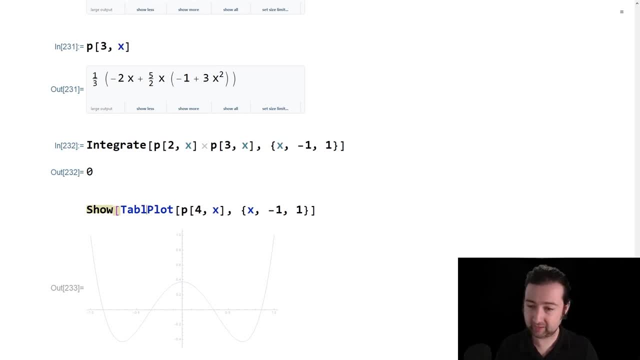 if we showed a table- That's a cute trick- Show a table of plots where we're going to plot them all on top of each other. That's why we're using a show command here, And let's make this an? n, And then maybe we will evaluate our table from. 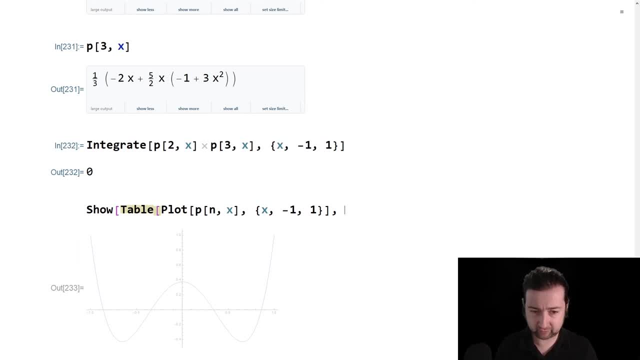 x, I don't know. n goes from 1 to 5.. Let's look at the first five Legendre polynomials plotted together. Well, that looks great, but not very satisfactory because they're all the same color and that's kind of jumbled. 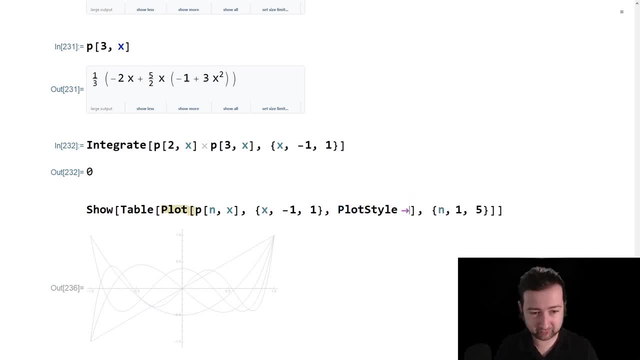 So what I could do is- and we've used this trick before as well- we can actually just make sure that each individual plot has a different color by using some kind of command that looks like this: And now we're going to get a family where each member of the family has its own color. 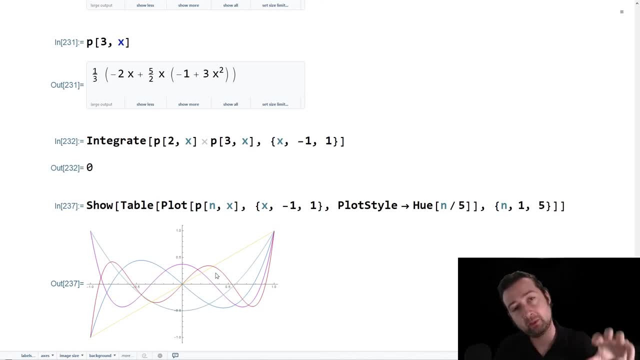 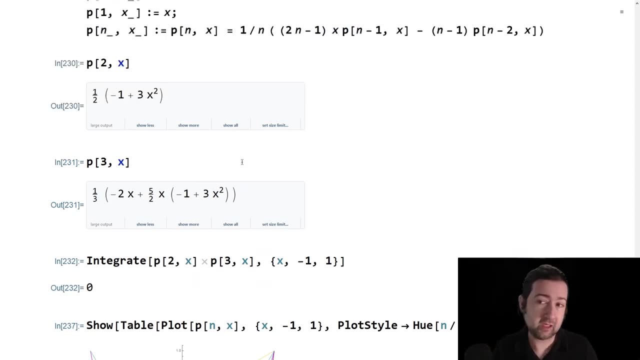 OK, so the whole point of this exercise is to show you that when we're working with these recursively generated functions, they are actually just functions and that you might have to do a little work on the relation to make sure that you get the right kind of equation. 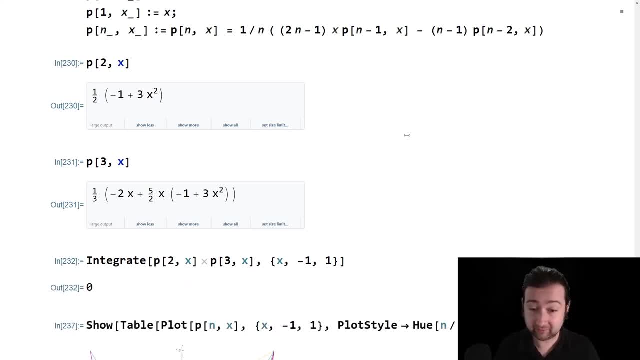 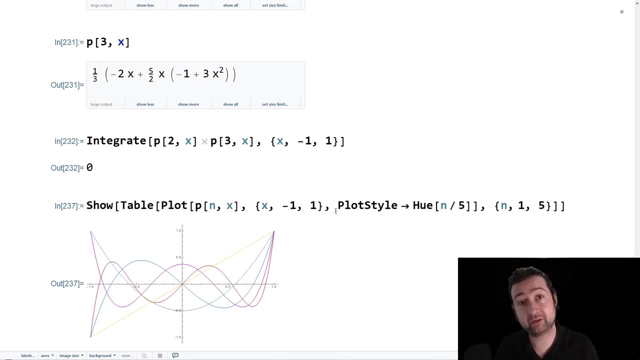 for relating these things. But once you have it, you just have functions, families of functions. In fact, there's an entire theory of using these functions to do approximation that shows up in linear analysis. that I think would be very appropriate to approach with Mathematica or MATLAB. 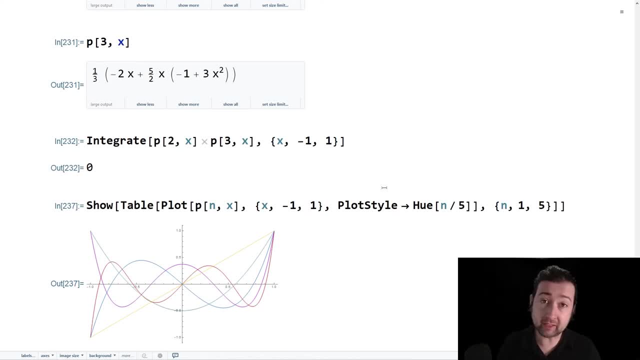 where you could actually see how these things work and why they're useful. So that's the basics of recursion. We talked about doing recursion to generate sequences of numbers. We talked about doing recursion to generate sequences of functions different ways that we can make sure that we have functions versus numbers. 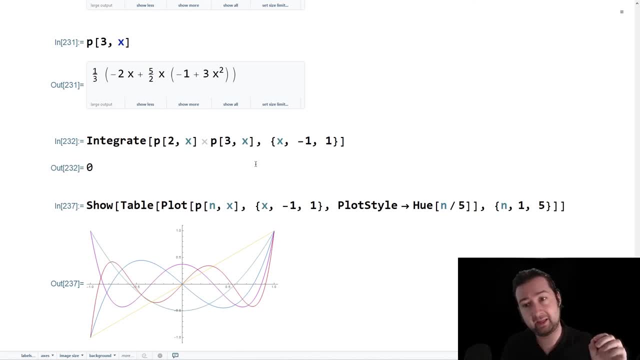 We've shown how we can manipulate the output of these things And we've also shown- even though it's not called this in the book- the idea of memoization, which means that you save the evaluations that you've already made so that you can call on those evaluations in the future.